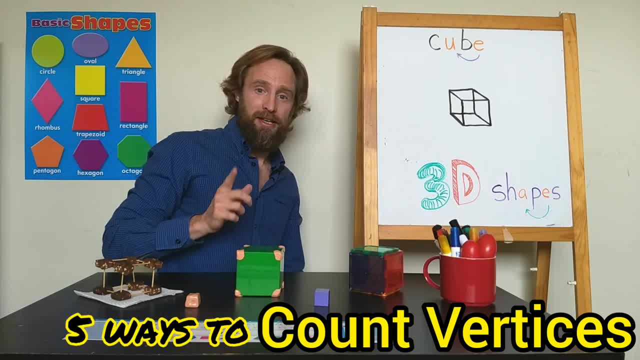 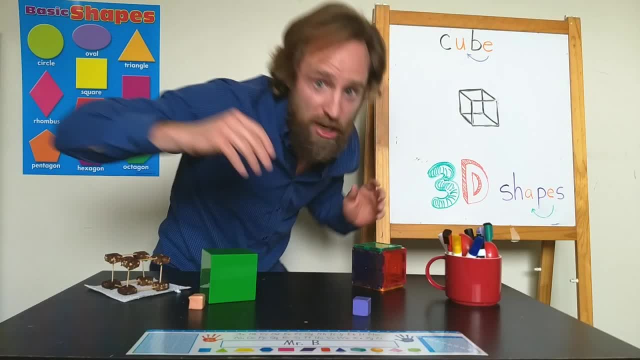 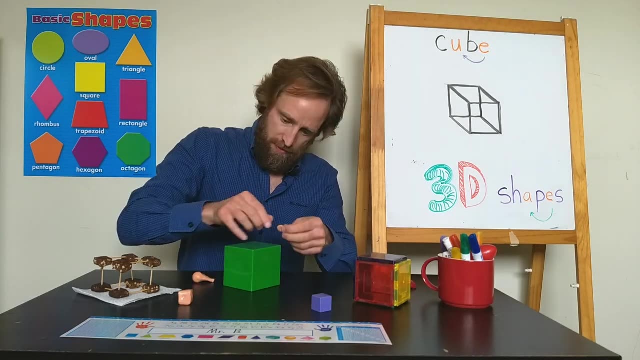 Today I want to tell you five fun ways that you can count vertices on 3D shapes and it's going to be more meaningful to the kids. Let's get started. 3D shapes coming at you, Get yourself a solid and get yourself some dough, clay or putty. You actually take this and put a little. 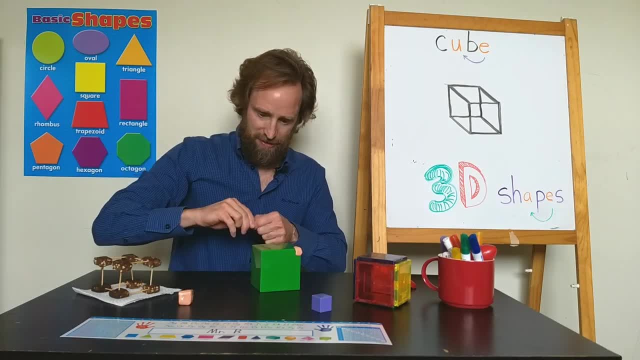 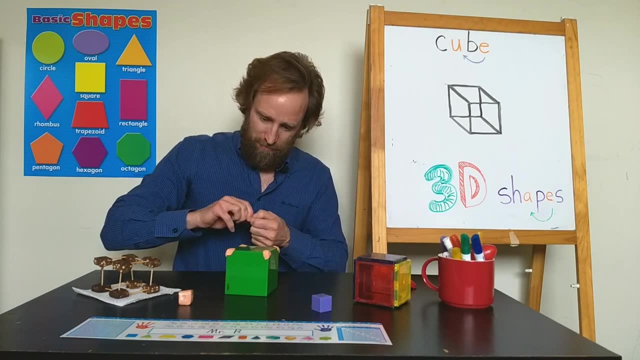 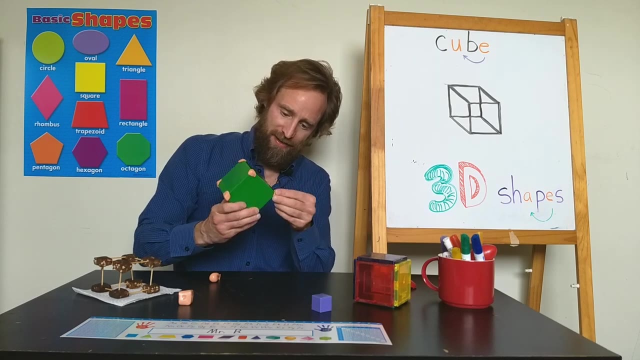 putty on every vertex. Just feel that point and really get an understanding what vertex means. It's a pointy part, but they're going to have a highly visual. Look how much that pops out, that putty. That is jumping out at your eyes and they're feeling it every time they put it on. 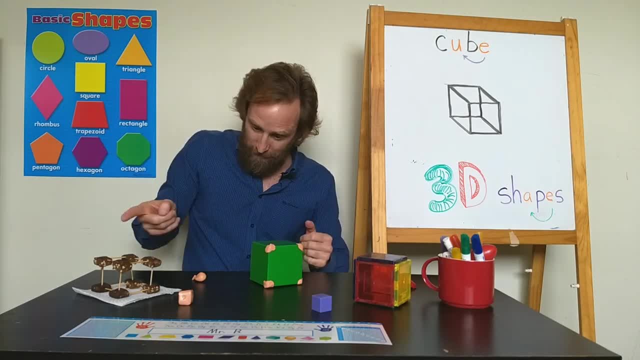 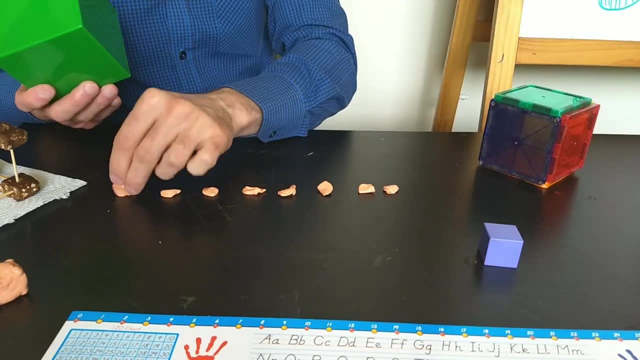 They can count as they put it on, count as they take it off and count as they line it up. You can lay them out: One, two, three and eight. There's eight, and I'm looking at the cube. There's. 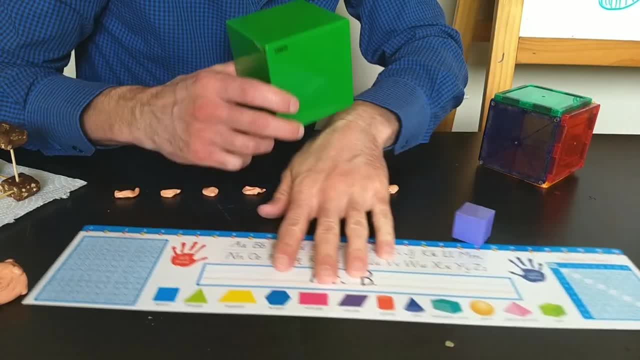 none left, so that way I'm not double and triple counting On 2D shapes. you'll know they'll go one, two, three, four, five, six, seven, eight, nine. You've seen it happen. Imagine how hard it is. 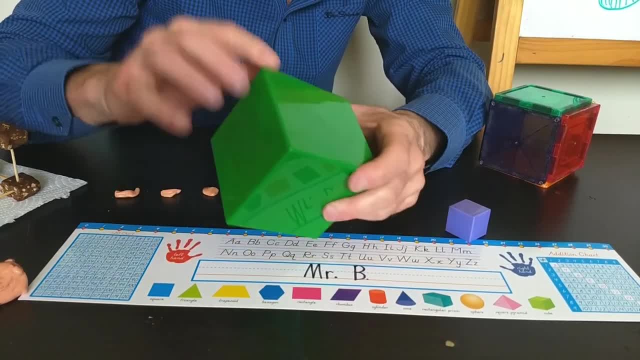 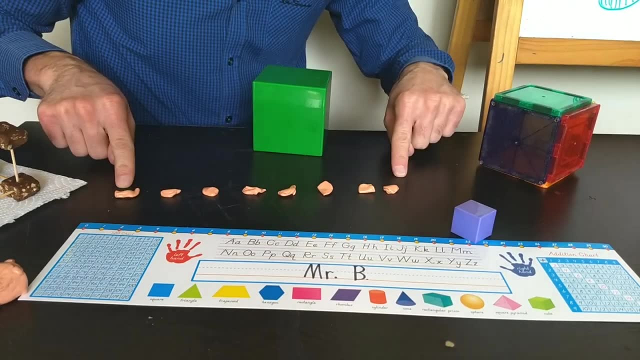 to keep track of which vertex you've counted here: One, two, three, four, five, six. Uh-oh, where did I start? Where did I stop? I have no idea. This will help you keep track. Coming down here for our. 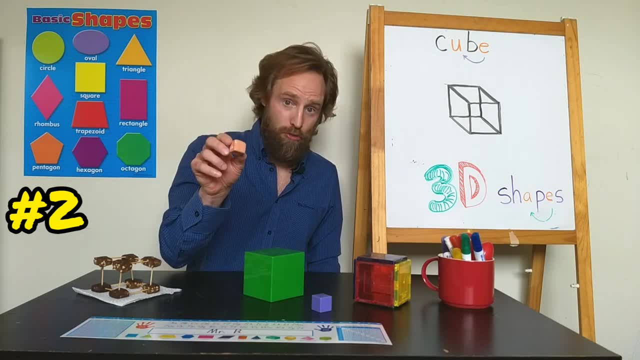 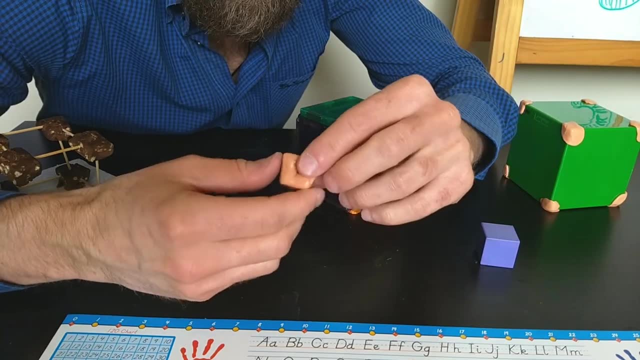 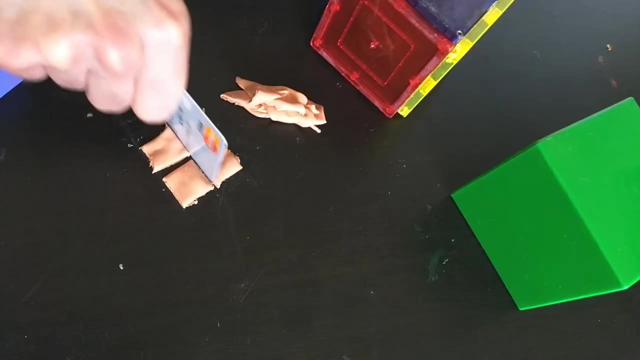 art-minded students. you could have them construct their own cube with a putty or a dough or a clay. I've crafted the shape out of putty, which is great because it's going to show you this isn't a square. It's made up of six different squares. What you can do to emphasize the vertice or the 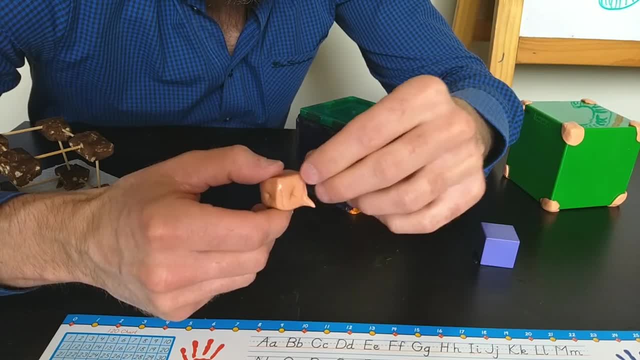 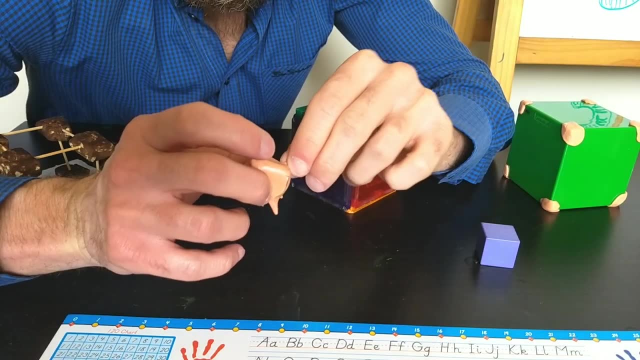 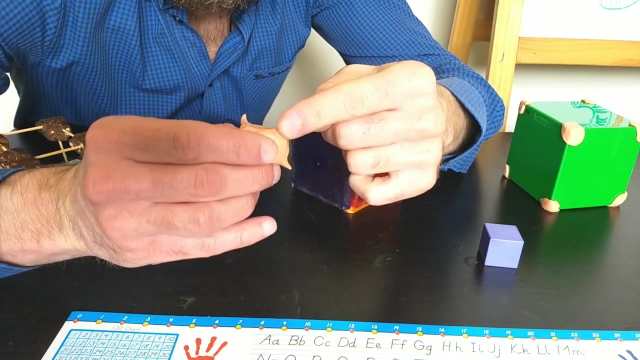 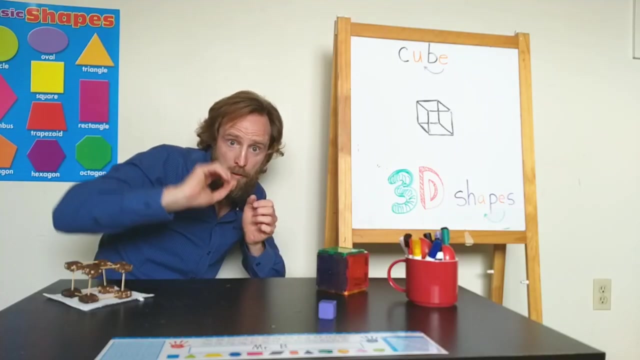 vertex is. pinch it, Make a little horn, And that's two. How many horns do you have to make? Oh my goodness, it's almost like a sea anemone. Try saying that one time, slowly, and I can even push it to recount: One, two, three, four. You get the idea. 3D shapes: Don't ever throw stuff at the 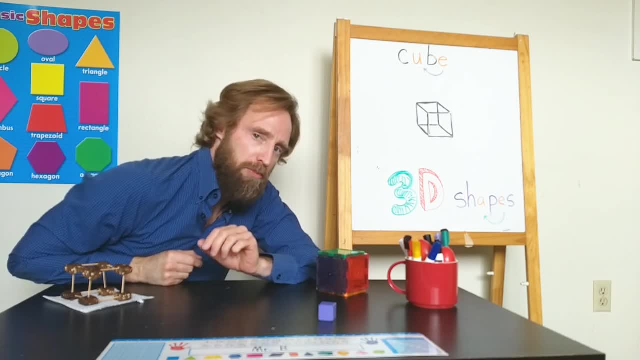 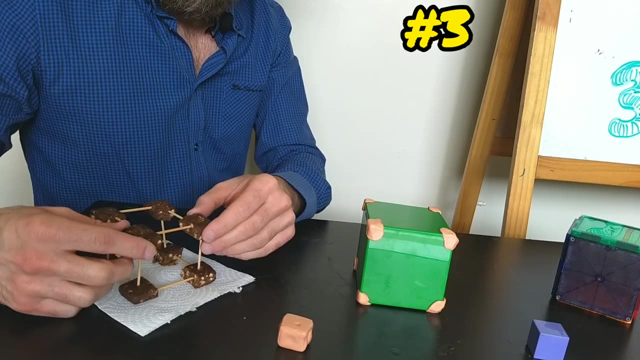 camera. I only did it because I'm a trained expert. I could have been a professional baseball player And you know what baseball players throw Spheres. As you can see, this is for your builder. It's hands-on and it's actually tongue-on. You can use your sense of taste, because this is made out of. 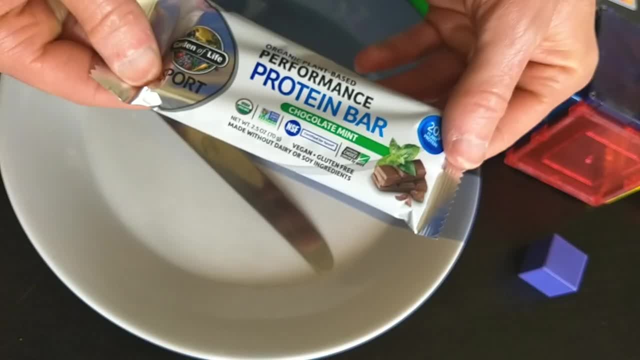 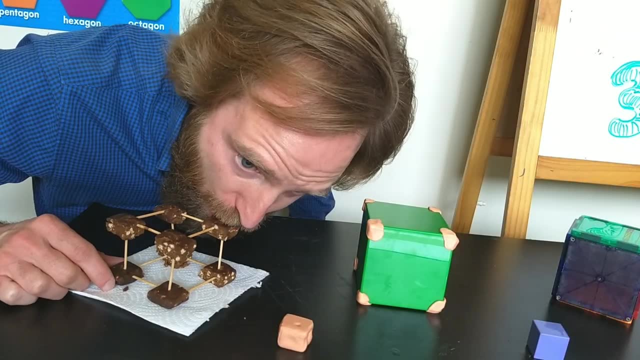 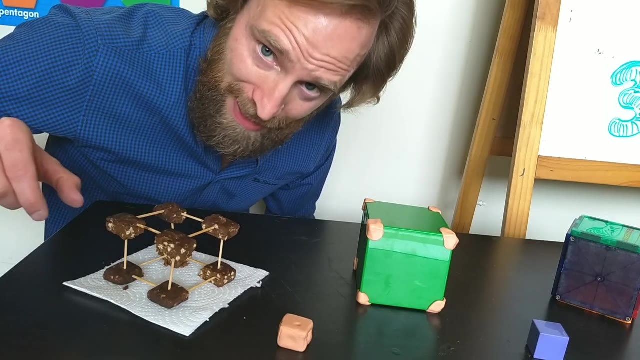 edible materials. Now I say, use your protein bar And then you can count as you eat How many vertices A lot. Don't eat it because I'm still doing the video. Okay, I'll eat it later, But I could pick these off, lay them out, count it. 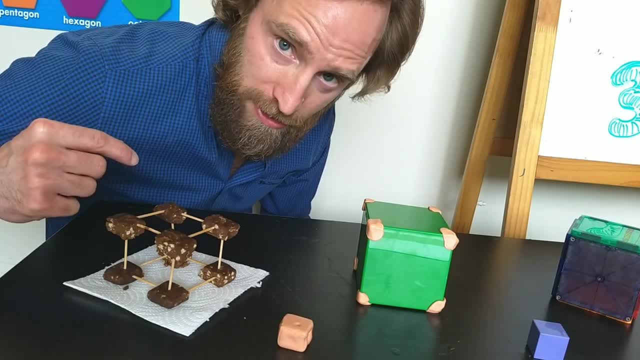 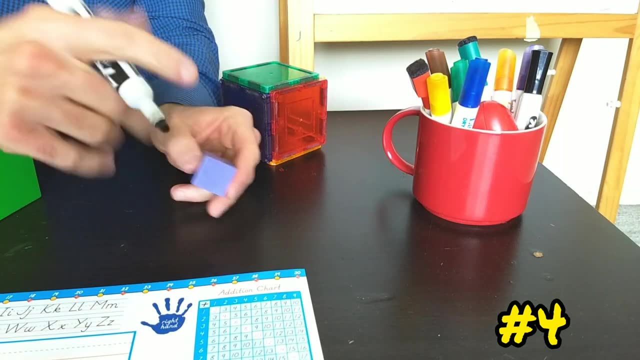 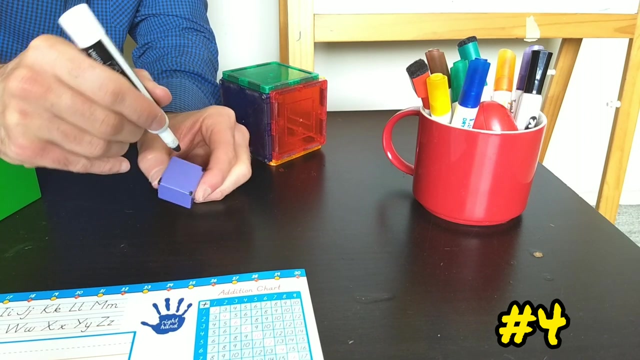 and then count again as I eat them and get my nutritious, protein-laden, nutrient-dense snack. Moving to the tiny cube, Take the marker and again, in the name of keeping track, Nice Black mark. there There's one, two, three, four. That's a good way so they don't double count, or? 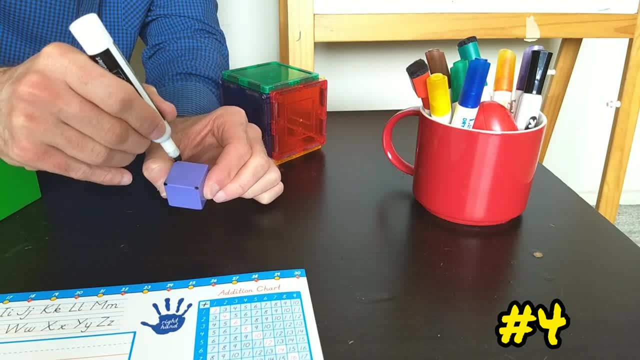 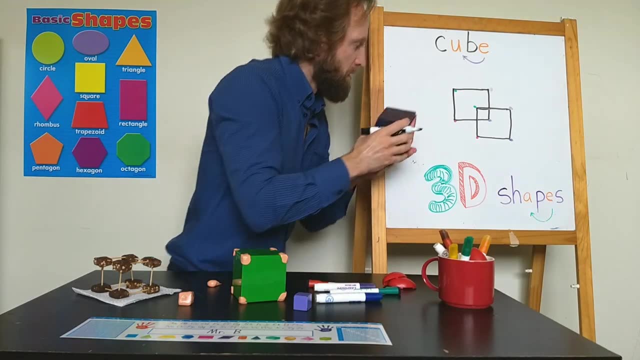 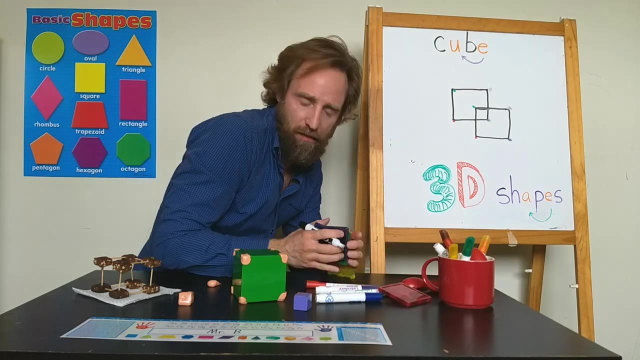 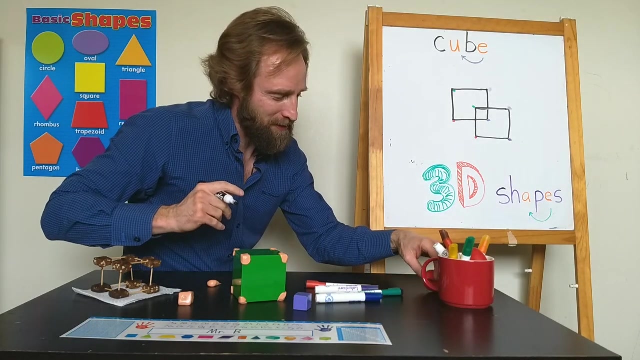 undercount And once you have every black mark on and you count at eight, you can double check by erasing One, two, three. See if I can do this at the same time. Outtake: Everyone makes mistakes. You got to roll through them and keep on trucking. Get something that's transparent or translucent. 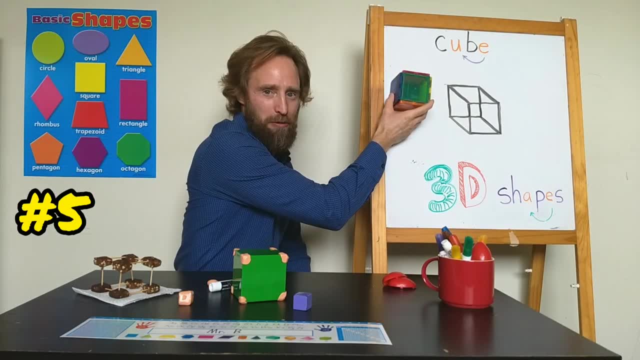 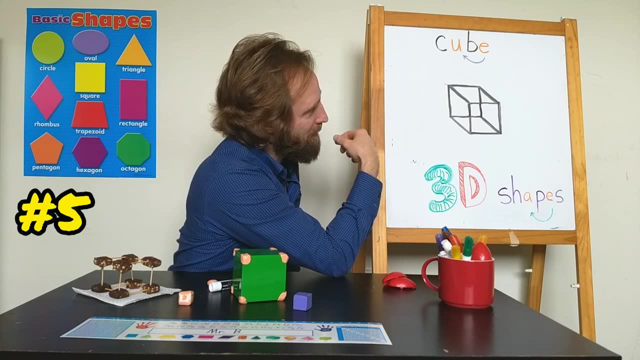 like a magnet tile and hold that right next to it so they can see what are you trying to depict. Because if you just show them this that is just going to look like a weird 2D shape to a small child, You have to show them where you got it from. So, as a matter of fact, 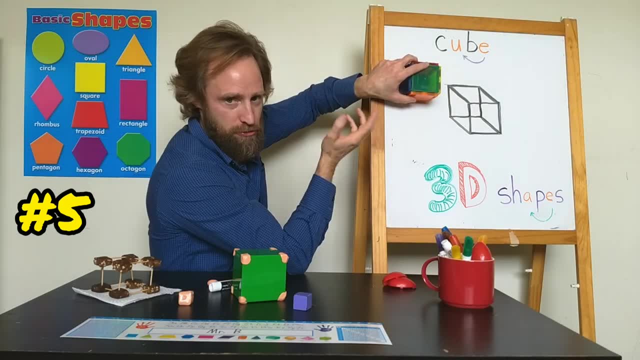 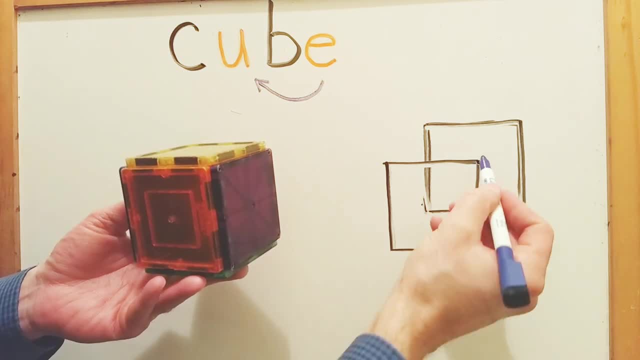 you can hold this up as you show them how to draw it, or as you show them the 2D picture And, better yet, have them make it, If the child can play, connect the dots, lay out some dots- Blue, blue, Red, red- And as you're. 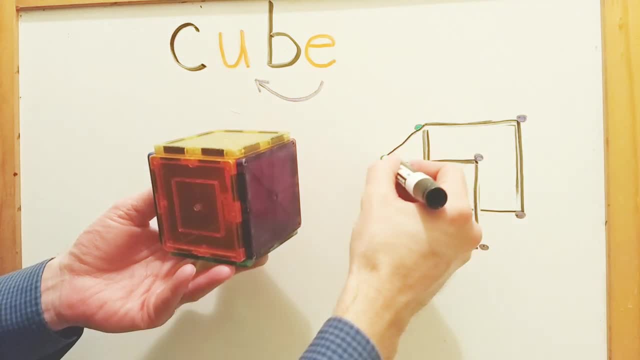 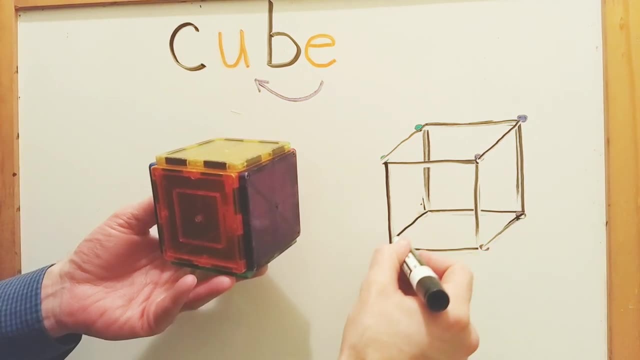 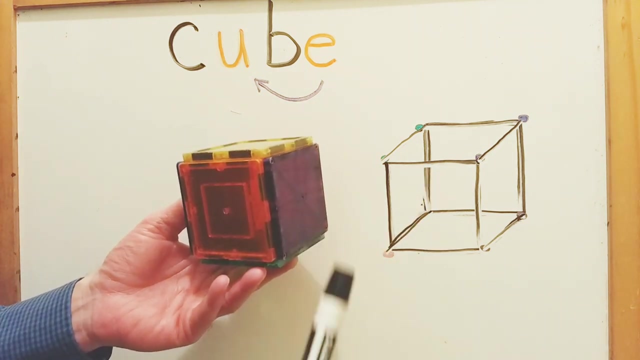 holding this and they start connecting it. hopefully they have that aha moment They go. oh, you weren't drawing a crazy hexagonal spider web. You were showing me a 2D representation of this cube. You can have a couple.